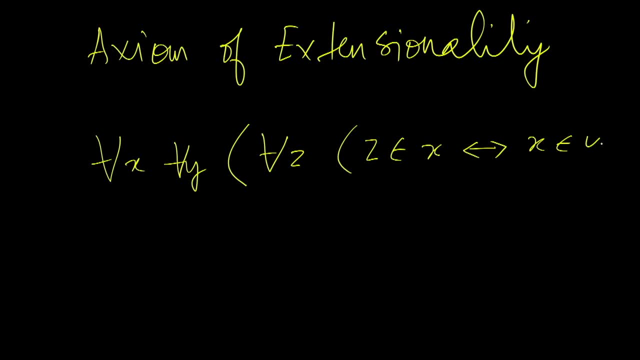 x if, and only if, z belongs to y implies that x equal to y For any two sets, x and y. x and y have exactly the same extensions, That is, the same z belongs to both of them for every z, in which case x is equal to y. This is the first axiom. 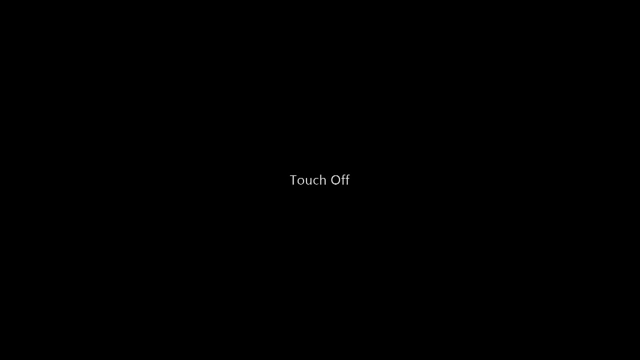 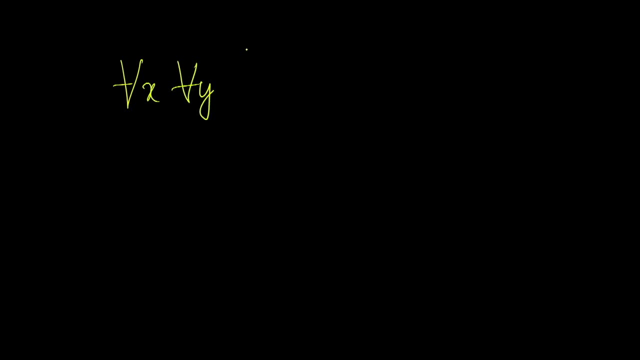 Now, for every x and for every y, for a pair xy of z, there exists z, So that for every u, u belongs to z if, and only if, u equal to x or u equal to y. In other words, for every pair x, y of z's there is a set z, so that something is a member. 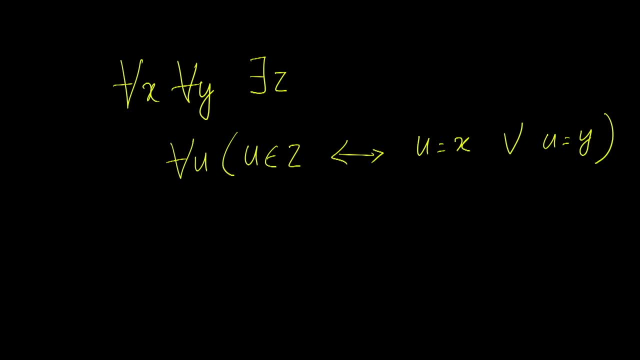 of z, precisely when that something happens to be either x or y. In other words, z contains exactly x and y and nothing else. The fourth axiom is the power set axiom. Power set of x, we know, is the set of all subsets of x. So the power set axiom asserts the existence of a power set For every set x. 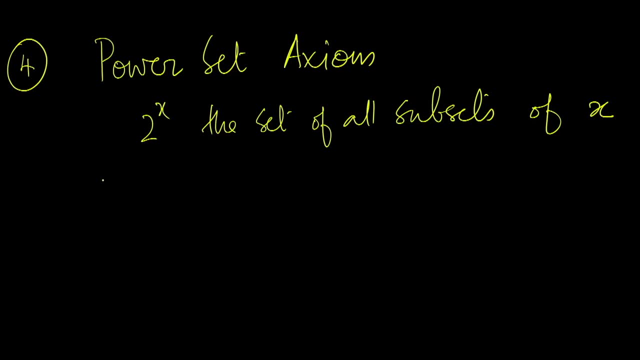 there is a set which happens to be the power set of x. In other words, for all x there, x is a y which happens to be the power set of x. So how do we state that We have to say that for every z, z belongs to y, precisely when z is a subset of x, In other words, z. 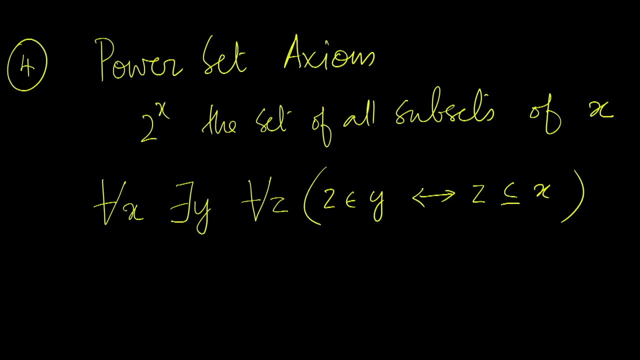 is a member of y precisely when z happens to be a subset of x. So all z affects or y will contain precisely the subset of x or y is the power set affects. So axiom-4 asserts the existence of the power set for every set. The fifth axiom is the. 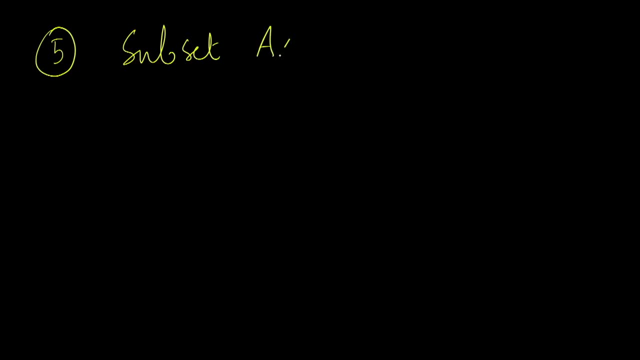 subset axiom. This is in fact an axiom schema For a formula, alpha with its free variables among t 1 through t k, y and u. So alpha is a formula with free variables. among these we have this following axiom: For all t 1 through t k, for every tuple t 1 through t k and for every: 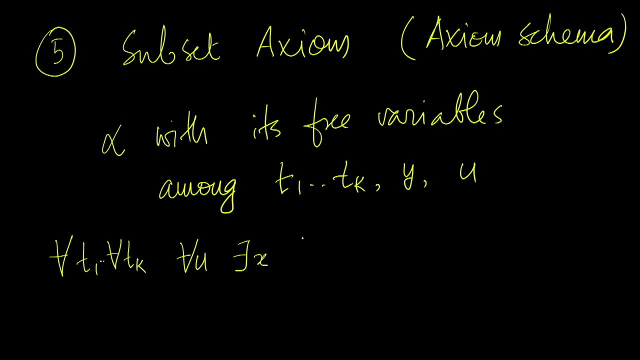 u. So x is an x, so that for every y, y belongs to x if, and only if, y belongs to u and alpha of t 1 through t, k, y, u is true, But if you replace any power over y, you get. 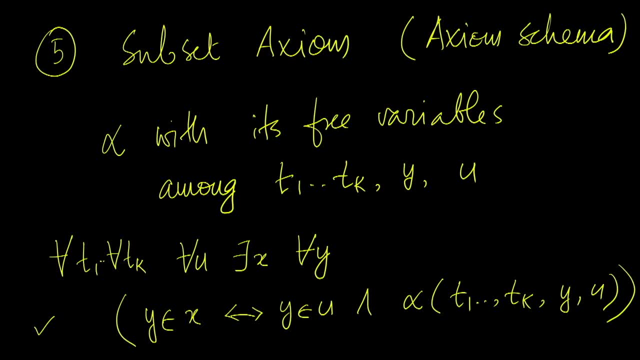 1. t 1 through t k y u alpha will be same for every formula alpha with its free variables among t 1 through t k y u. So when t 1 through t k y u are supplied as arguments, 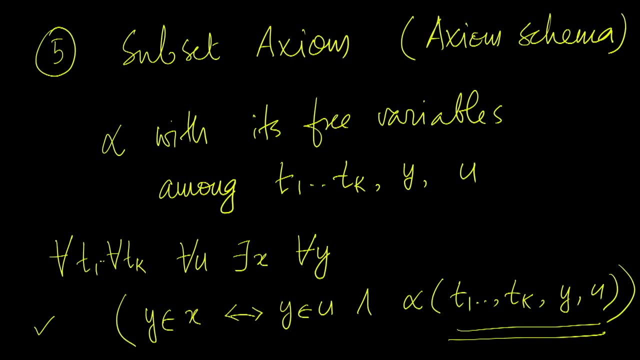 to alpha, you have to perform the substitution. if one of them happens to be the free variable, For example, if t 1 is not a free variable, then the argument which is supplied here will not be substituted. So what does it say? What it says is that, given any i thumb of 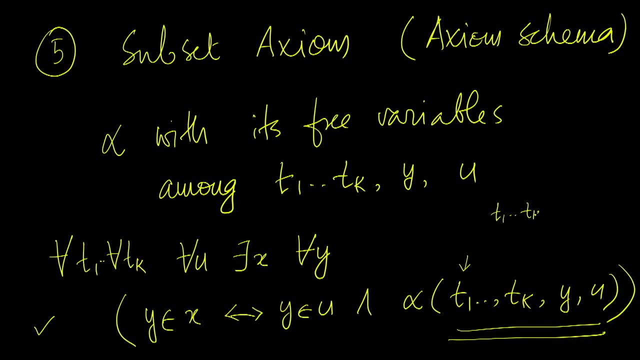 Given any k tuple, t 1 through t, k and a set u, then we can pick out the members of u which satisfy the formula alpha, along with y and u with t 1 through t k. In other words, given the tuples- tuple t 1 through t, k and u, there x is an x, a set which we can synthesize from. 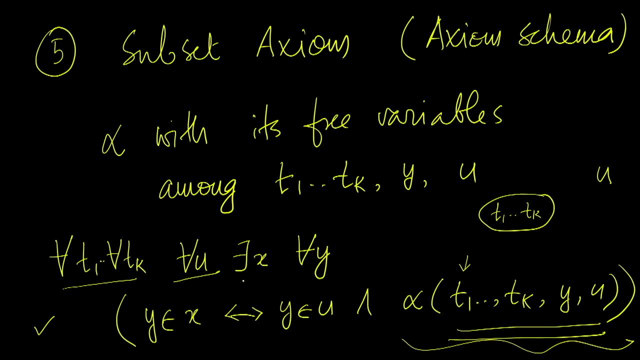 u and t 1 through t k, so that membership in x of y will be precisely when y is a member of u. In other words, x will be a subset of u. So we are forming a subset of u. x is. 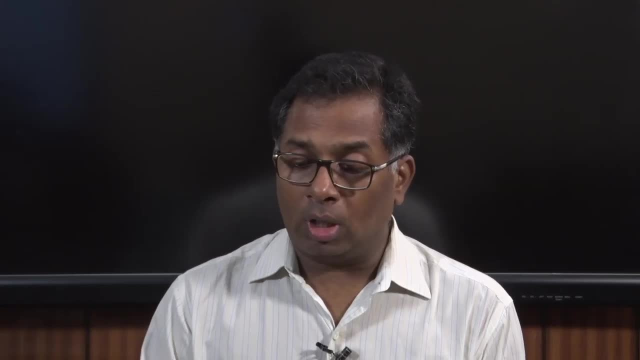 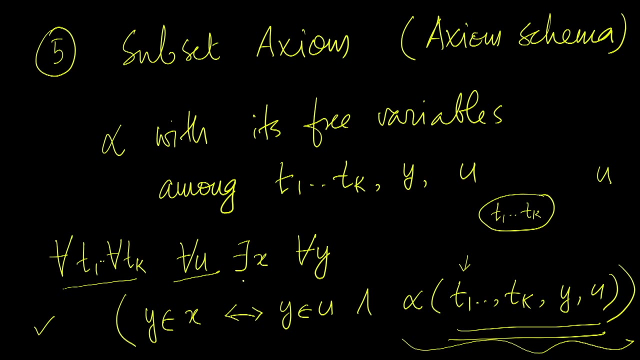 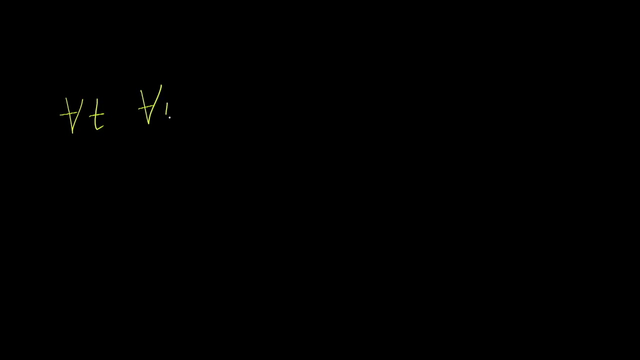 a subset of u And, moreover, u and y will have to satisfy the condition alpha, along with t 1 through t k. This is a way of forming subsets of a given set u. An example would be: for all t, for all u, there x is an x, so that for every y 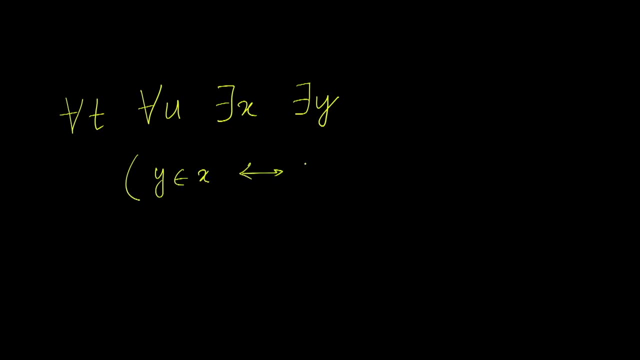 So y belongs to x precisely when y belongs to t and y belongs to u. Now, what does this assert? There exists the intersection of t and u, So for every set u when t is supplied, t is a subset of u. 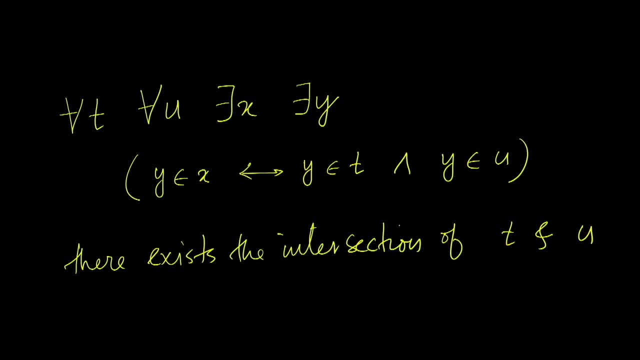 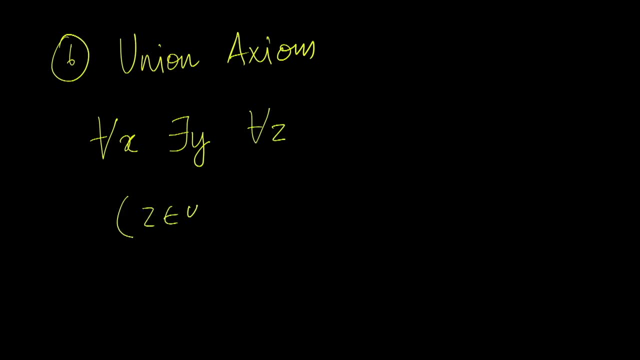 For every z, z belongs to y, precisely when there exists a u, so that z belongs to u and u belongs to x. Or, in other words, given any set x, we can construct a set y which will contain precisely the members of members of x. that is, for a z to belong to y that will have to belong to some u which. 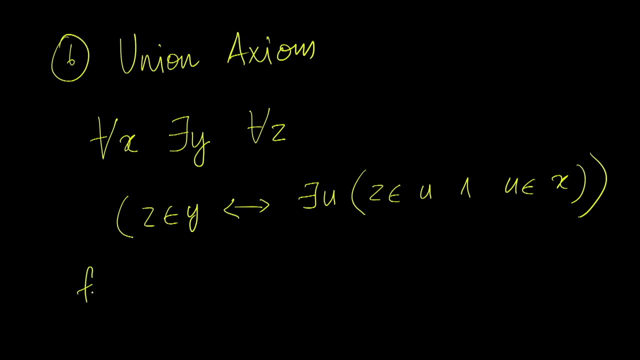 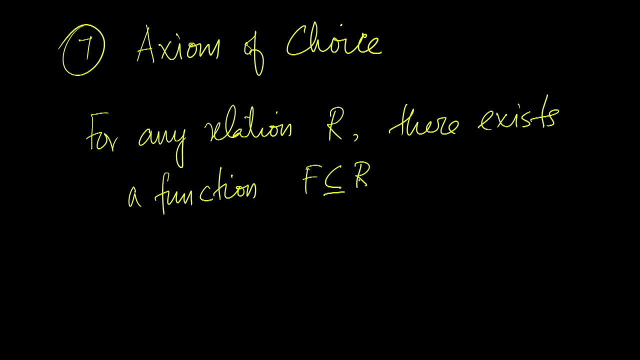 in turn belongs to x. So for any x there is a set y that contains precisely the members of members of x. The seventh axiom in our list is the axiom of choice. Axiom of choice says that for any relation R, there exists a function f which is a subset of R, such that the domain of 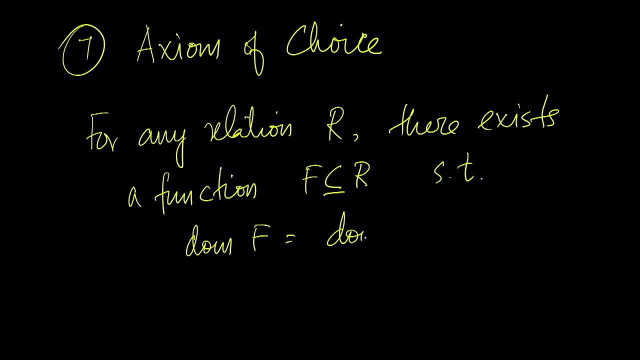 f is the domain of R. Why is this called the axiom of choice? Given a relation R, let us say from a to b, therefore this is a subset of a cross b. then consider some member x of a. under the relation R, x may have two images. let us say y 1 and y 2. 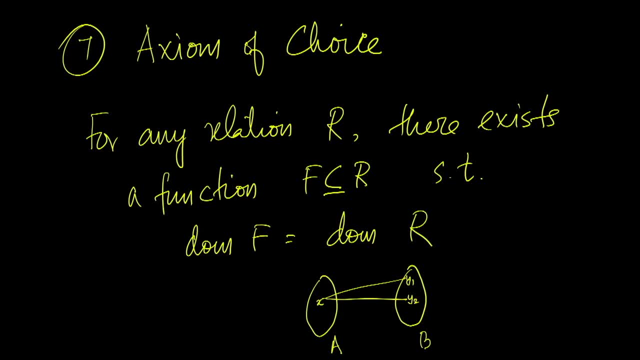 But what we construct here is a function, the domain of which is identical to the domain of R. therefore x will have to have an image under f as well, But then x has two images under R to form f. you will have to pick one Axiom of them, that is, you have to exercise the choice y 1 or y 2. one of them will be: 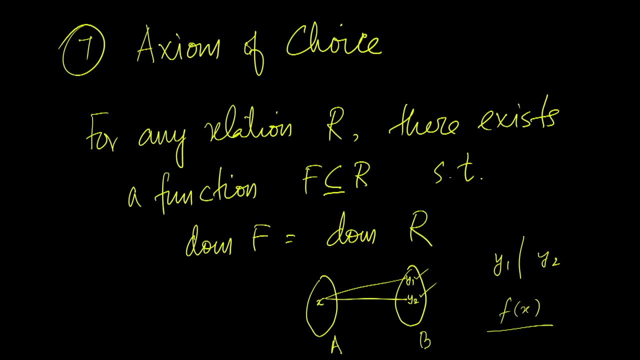 f of x for the function f that we are going to construct. Therefore, we are exercising a choice when we construct function f. So what axiom of choice says that for any relation R, there exists a function satisfying this condition. that is the domain of the function. 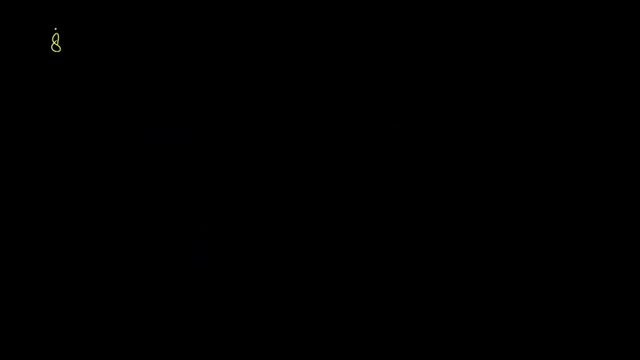 is identical to the domain of R. The eighth axiom is the infinity axiom. What this says is that there is an inductive set, or formally, there x is an x, So that the empty set belongs to x And x is closed under the successor operator for every y. if y belongs to x, then the successor. 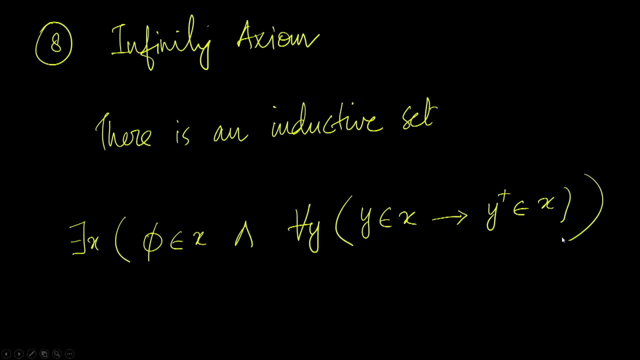 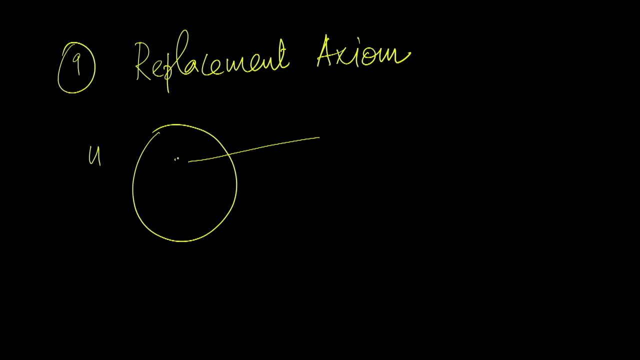 of y also belongs to x, that is, when x is closed under the successor operator. So the infinity axiom says that there is an inductive set, And the ninth axiom is the replacement axiom. Consider set u. suppose every member of u has a nominee n of x. 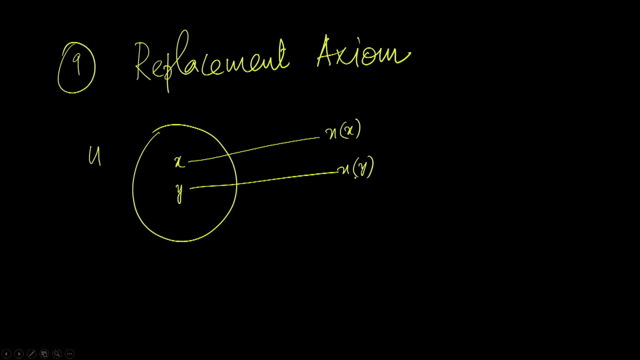 For the y, the nominee is n of y, So the nominee function defines a unique nominee for every x. Then What this axiom says is that if every member of U has a nominee, then there is a set that contains precisely the nominees of the members of U, or in another words, for any formula. 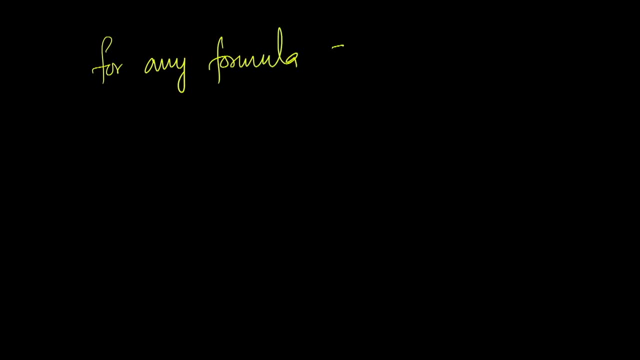 typically nu of x, y, which in fact asserts that y is a nominee of x, in which z is not free. The following is an axiom for every u for all x belonging to u for all a and b: nu of x, a and nu of x b implies that a equal to b. 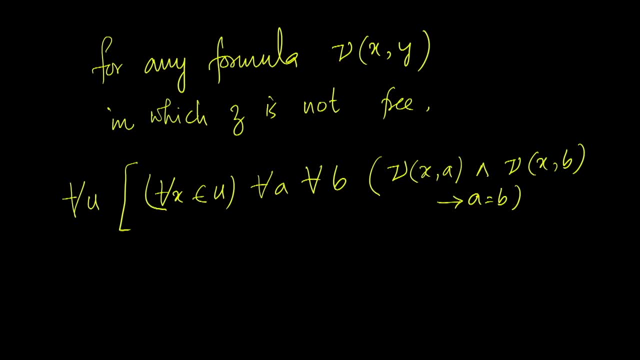 So this is the antecedent of an implication. What this says is that for every a, b, nu of x a and nu of x b implies that a equal to b, In other words, there is exactly one a for every x, so that nu of x a is satisfied. In other words, x has a unique nominee. Then 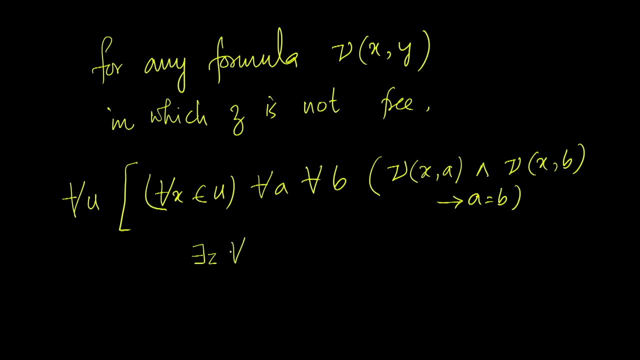 The rex is z, so that for all y, y belongs to z. if, and only if, the rex is x belongs to u, so that nu of x, y, In other words, the rex is a z which contains exactly the nominees of the members of u. 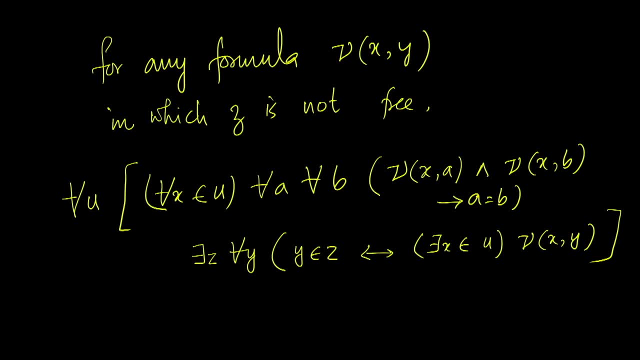 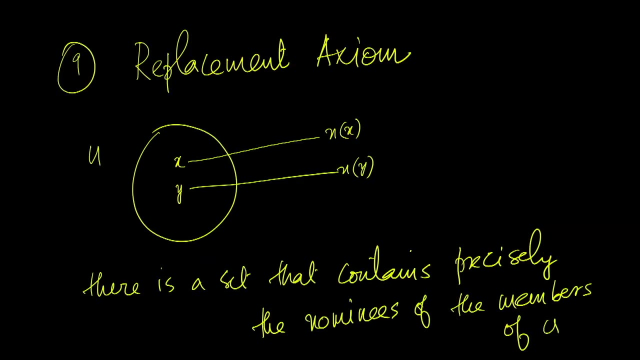 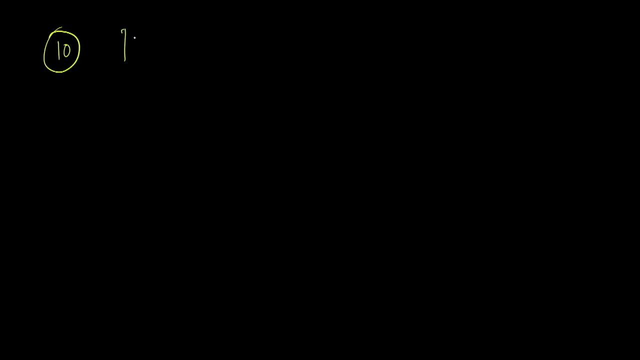 So for every y, y belongs to z, precisely when y is the nominee of some x, which belongs to u. So the assertion is exactly that we had in mind. There is a set that contains precisely the nominees of the members of u, And the final axiom is the regularity axiom. 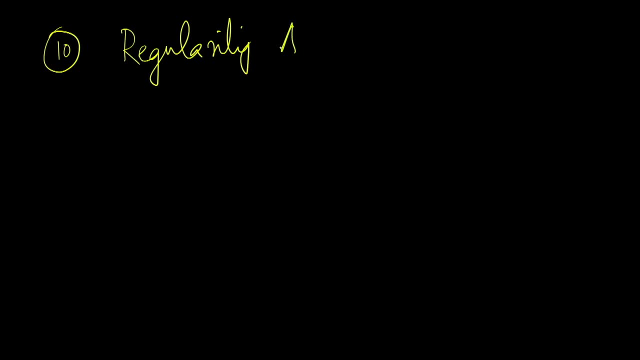 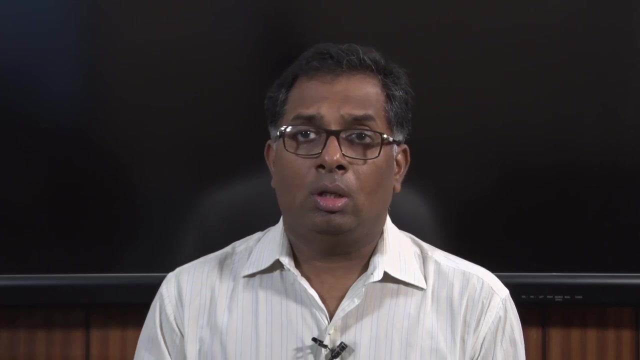 This says that very non-empty set x has a member y. with x intersection y equal to phi, you can show that this implies no set is an element of itself. The paradoxes that are known within naive set theory will not arise within Zermelo-Fraenkel. 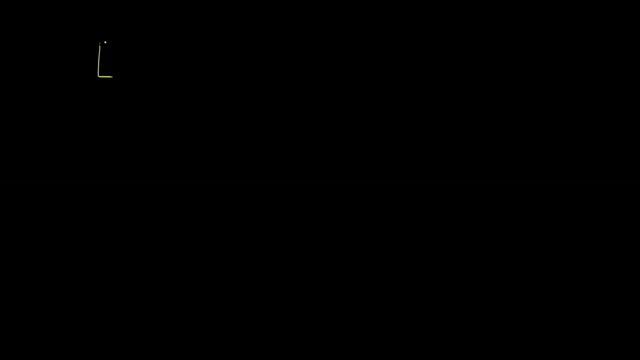 set theory. Now let us consider the notion of equinumerosity. We say that set A is equinumerous with set B. denoted in this fashion, A is equinumerous with set B if, and only if, there exists a one-to-one. 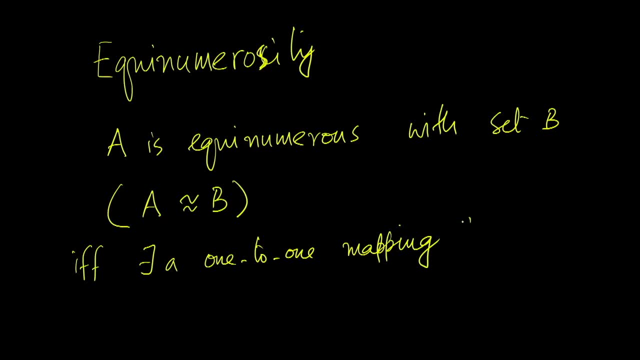 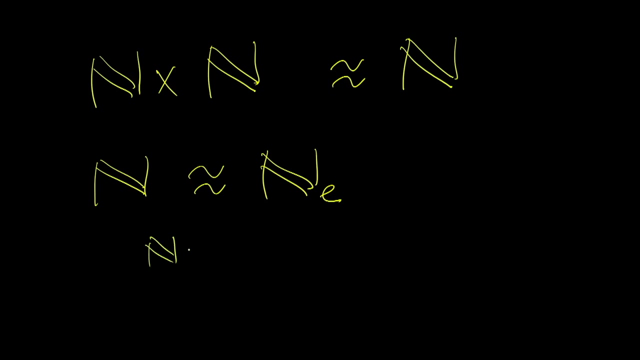 starting from A on to B, We have seen that n cross, n is equinumerous with n. The set of all ordered pairs obtained from n is equinumerous with n itself. Similarly, n is equinumerous with the set of all, even natural, numbers. n is the set. 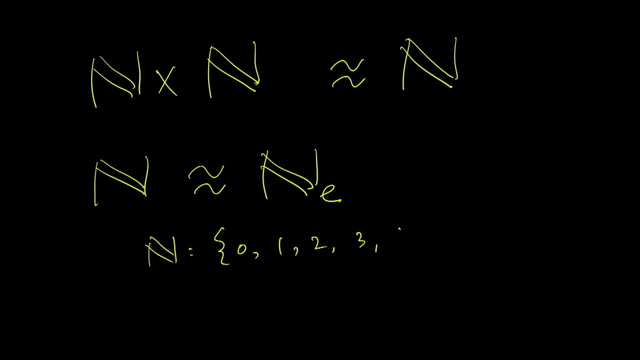 of all natural numbers, the set of all even natural numbers. Okay, So this is n? e. So there is a mapping from n to n? e, which is one-to-one and onto, in which we map x to 2 x. Coming to real numbers, we can show that the interval from 0 to 1 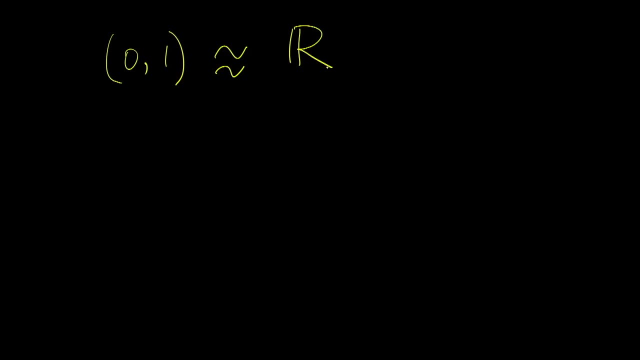 is equinumerous with the set of all real numbers. How do we show this? To show this, we consider the real line. Let us say: this is the origin and this is 1.. So we are considering the set of all points from 0 to 1 on the real 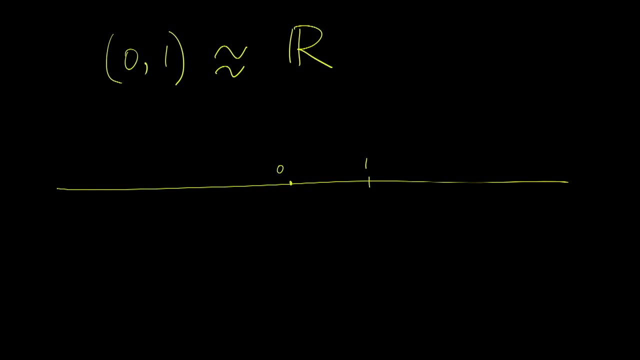 line. We want to show that this set is equinumerous with the points from the real line itself. Okay, So this is the set of all points from 0 to 1 on the real line. So we want to show: 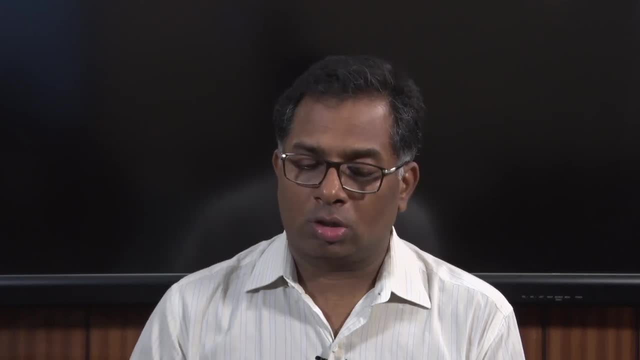 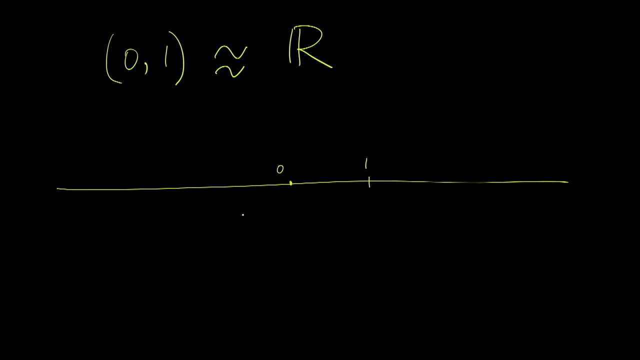 that this set is equinumerous with the points from 0 to 1 on the real line itself. To prove this, what we do is this: Consider the portion of the real line from 0 to 1, that is, a line segment from 0 to 1. We take it and bend it so that it forms a semicircle. 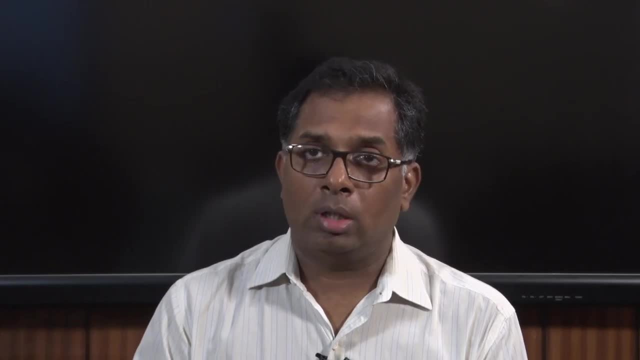 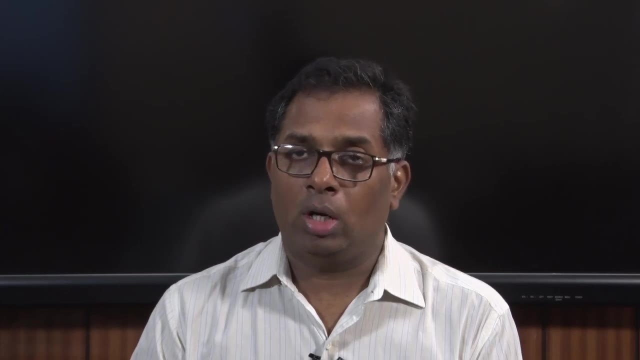 and arrange the semicircle so that the real line is a tangent to the semicircle. So the length of the semicircle is 1. Because this is the length of the semicircle. this is the length of the semicircle, So we want to show this as the tangent to the semicircle. So 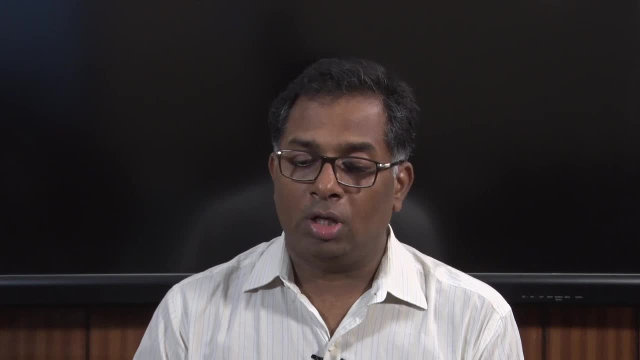 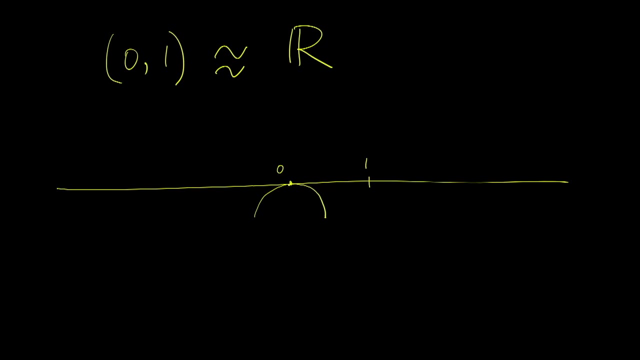 because this has been obtained from the interval 0 to 1 by bending the interval 0 to 1. So this has a radius of 1 by pi. So the origin of the circle would be 0 minus 1 by pi. on. 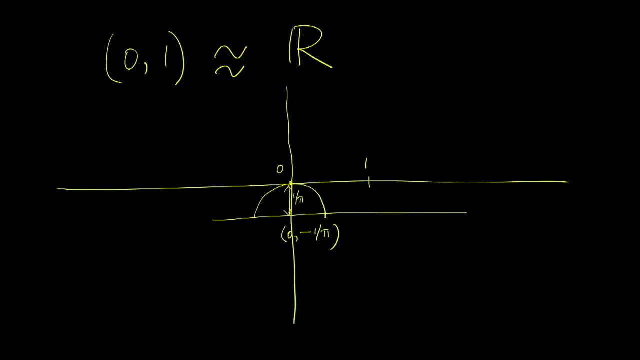 the real plane. So this is what the origin is. And then let us say we draw a line passing through the origin of the circle and some point on the real line. This ray, the ray with the origin as its, The vertex, will intersect the semicircle at some point and it will intersect the real 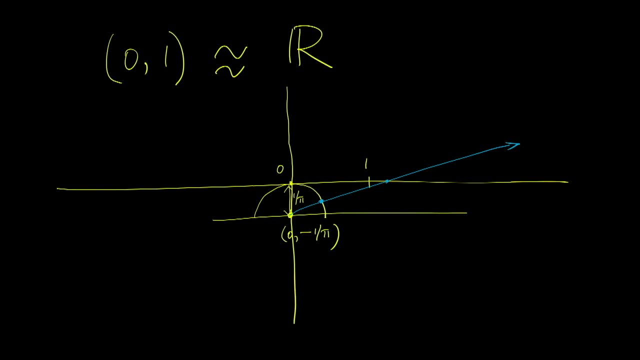 line, exactly one point. Then let us define a function f which maps the circle point onto the real line point. So f is defined in this manner. So this function f, This function f maps the interval 0 to 1 onto the real line, which is the set r. Consider: 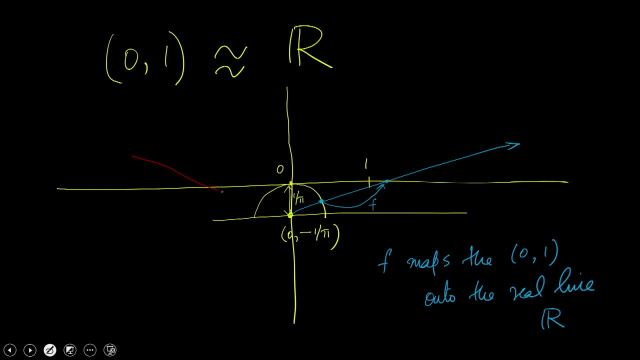 another line, for example, this will pass through these two points. So this point is equal to map to a negative real number. So it shows that the interval 0 to 1 has a 1 to 1 onto mapping to the set of all real numbers. Therefore the interval 0 to 1 is equinumerous with the 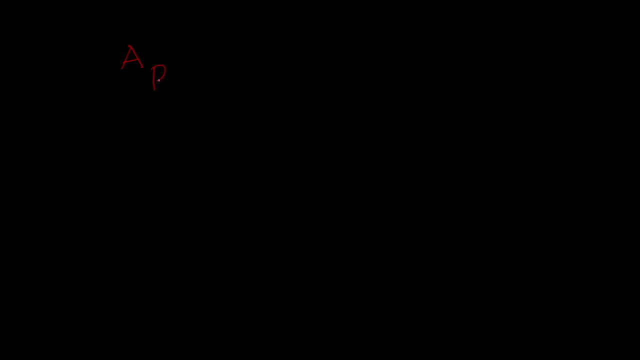 set of all real numbers. Let this be the notation for the set of all functions from A to B. In particular, A 2 will denote the set of all functions from A 2, the set 2 which, according to our definition, is this: We are considering the natural number. 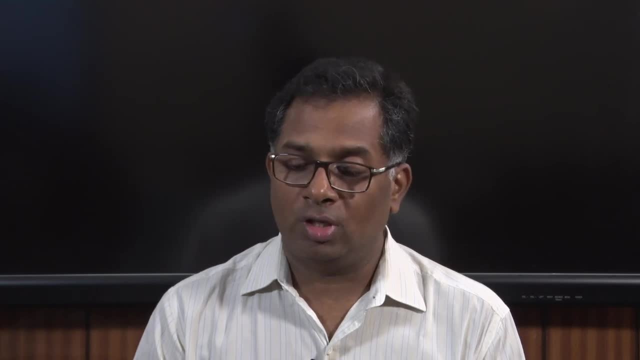 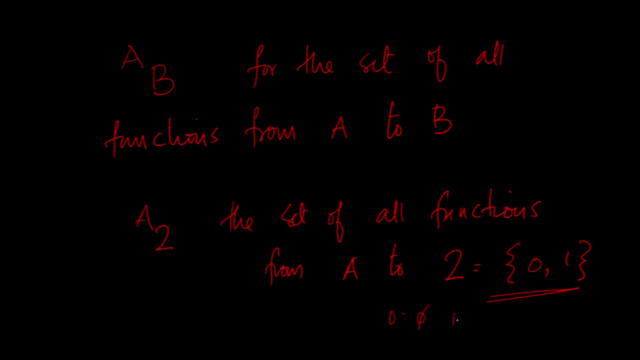 2. in the embedding of the theory of natural numbers in set theory we had defined natural number 2 as the set 0- 1, where 0 is the empty set and 1 is the singleton containing the empty set. So by superscript a 2 we denote the set of all functions from a to 2.. Recall. 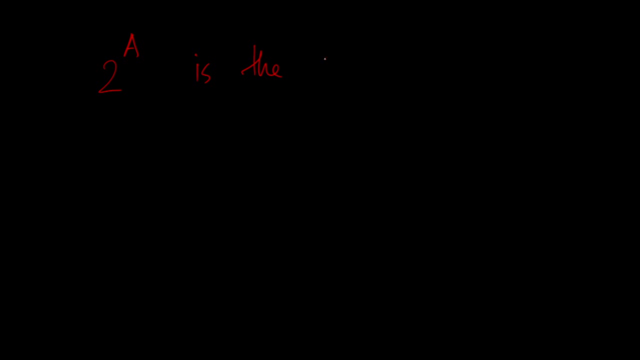 2. power a is the power set of a. We claim that superscript a 2 is equinumerous with 2 superscript a. This is the set of all functions from a to 2 and this is the set of all subsets of a. These two sets are equinumerous. 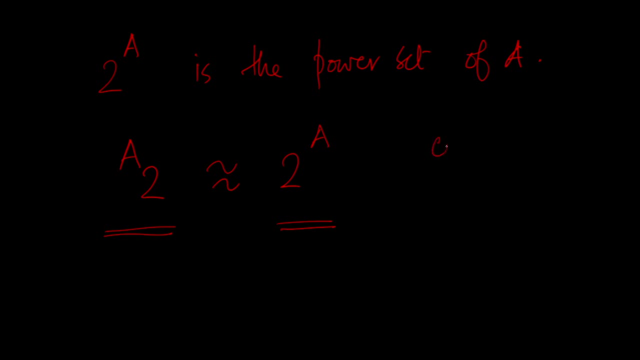 but how do we show that they are equinumerous? Let us consider any subsets of a. Suppose b is the subset, then b has a characteristic function, The characteristic function of b, f. b is defined in this manner: f b of x is 1, if, and only if, x belongs to b or in other. 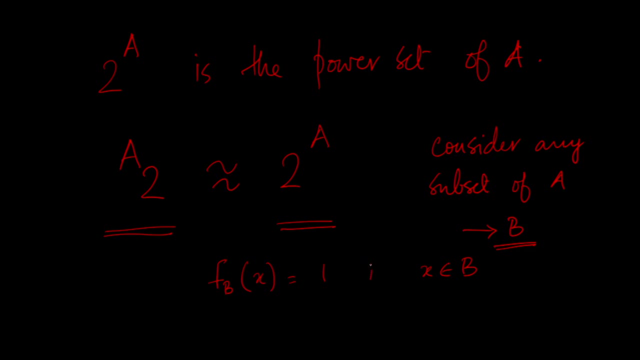 words: it is 1.. it is 0, otherwise The characteristic function is a binary function. So FB happens to be a mapping from a to 2.. So FB is a member of the set of all functions from a to 2.. So what? 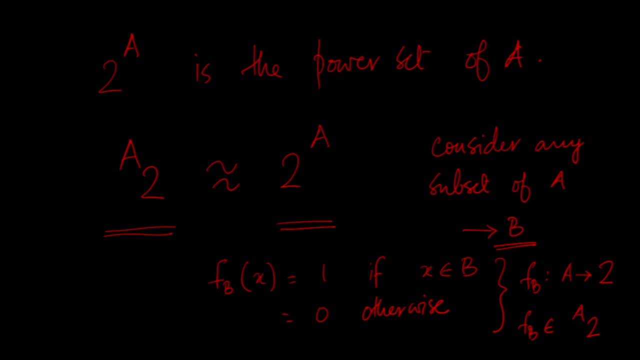 we find is this Corresponding to any subset B of A? there exists a unique function, FB, of superscript A 2, and this is a unique function. The characteristic function of B happens to be a member of superscript A 2.. Therefore, these two sets are equinumerous. 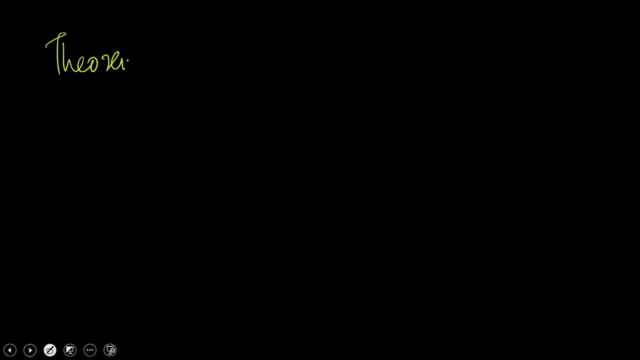 Consider a theorem. It says that A is not equinumerous with its own power set. No set is equinumerous with its own power set. How do we prove this? Consider any mapping F. Consider an arbitrary mapping F from A to 2 power A. So it maps the members of A to. 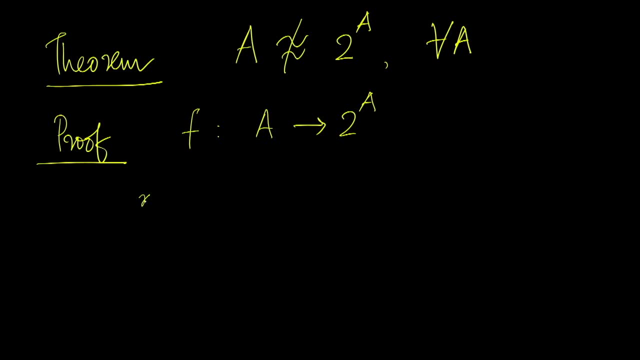 subsets of A. So for X, F of X is a subset of A when X is a member of A. So let us say that X owns the members of F of X. Then let us define a set, B. B is the set of, precisely. 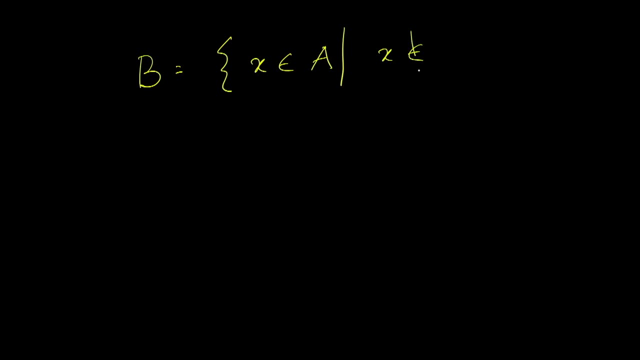 those members of A, So that X does not belong to F of X. In other words, B is the set of those members of A But do not own themselves. Then by definition, B is a subset of A. 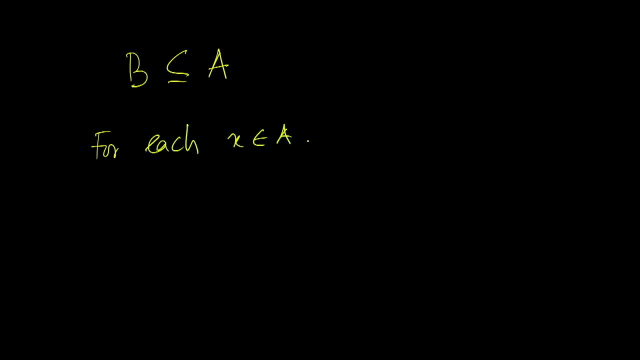 For each X belongs to A. X belongs to B if, and only if, X does not belong to F of X by For some x belonging to A, if B equal to f of x, suppose B happens to be the image of some x under f. then let us consider the possibilities. One possibility is that x belongs to B, but 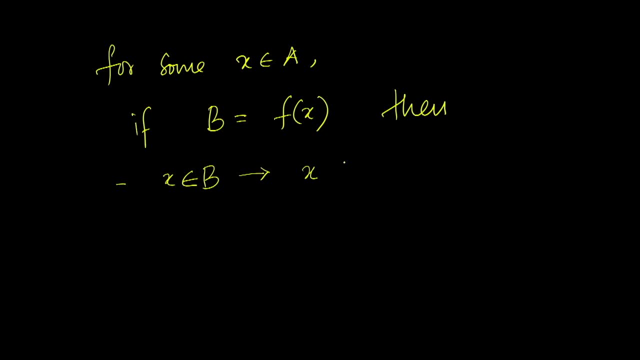 then B is the same as f of x, then x belongs to f of x. If x belongs to f of x, then x should not belong to B, Because B happens to be the same image of set of precisely those that do not own themselves. So if x belongs to f of x, then x owns itself. 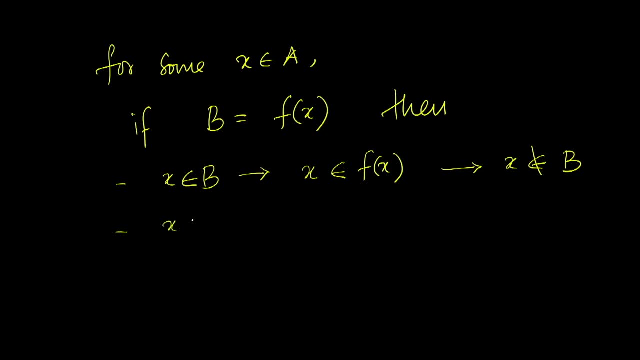 so x should not belong to B. On the other hand, if x does not belong to B, then x does not own itself. thus implies that x belongs to B. So either way we get a contradiction. Therefore, what we have 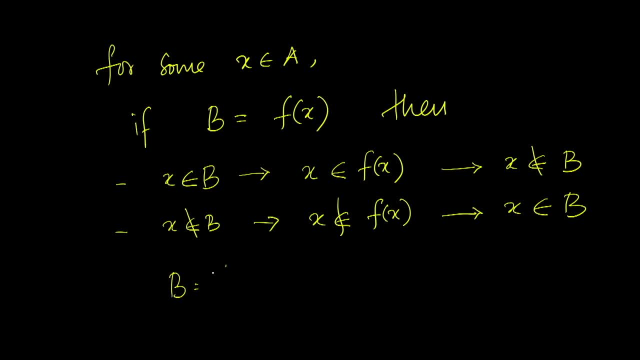 Is that B is not equal to f of x for any x, but B is of course a subset of A, which means B is a member of 2 power A. Therefore there is a member of 2 power A, Therefore there. 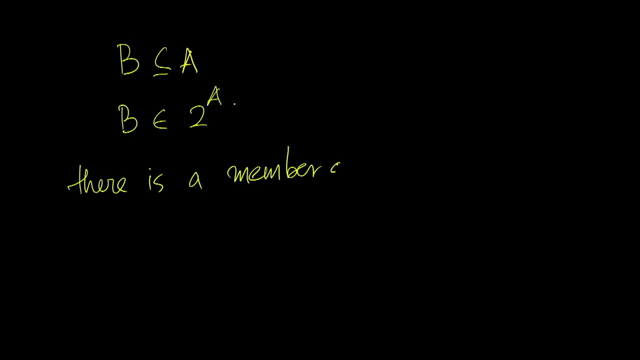 is a member of 2 power A. that is not an image under the function f, or in other words, f is not onto Mind you, the function f that we considered is an arbitrary function, So the function f is not an arbitrary function. 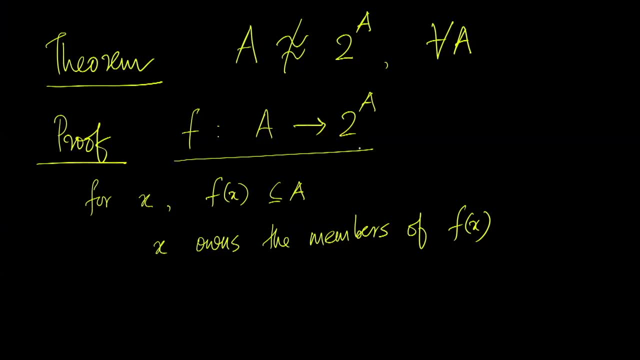 It is an arbitrary one. We have considered an arbitrary function, f, here, And what we have shown is that this function is not onto. So any function f from A to 2 power A is onto. So what we have established is that f is not onto. Since f is arbitrary, we have 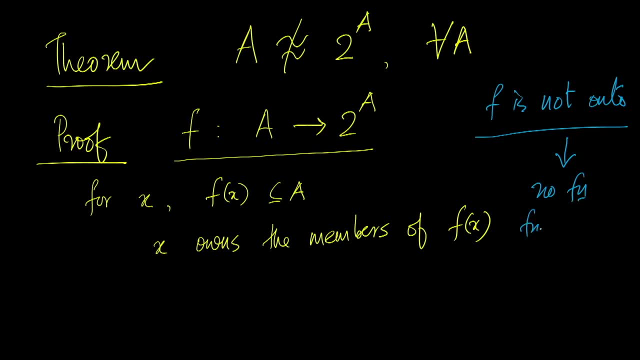 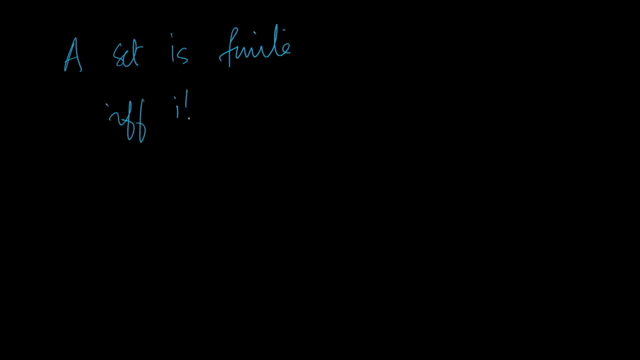 that no function from A to 2 power A is onto, Which means A is not equinumerous to 2 power A. In other words, no set can be equinumerous with its own power set. We say that a set is finite if it is equinumerous with its own. 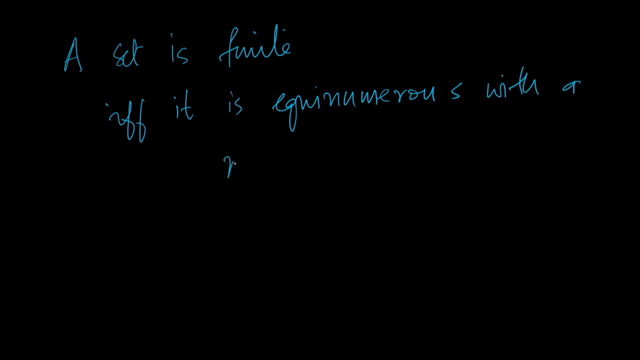 power set. So a set is finite if it is equinumerous with its own power set. So a set is finite if it is equinumerous with its own power set. Now let us consider a theorem which is famous under the name Pigeon-Holt principle. What? 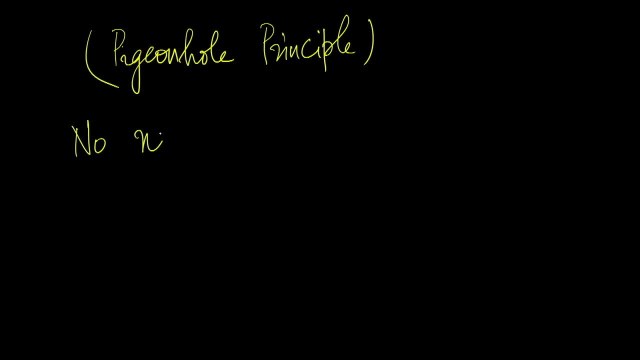 Pigeon-Holt principle says is that no natural number is one in all. So a set is finite if is equinumerous with a proper subset of itself. Remember n minus 1 is a subset of n under the definition of our natural numbers. So what it says is that no natural number is. 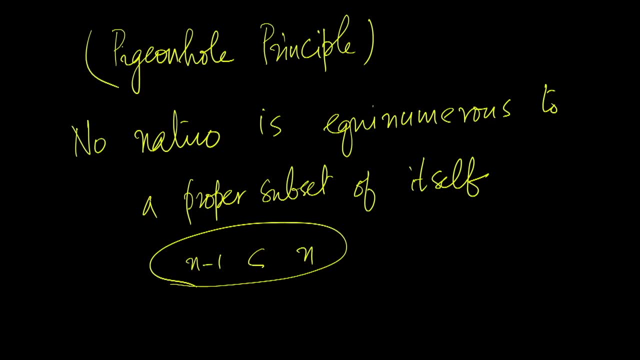 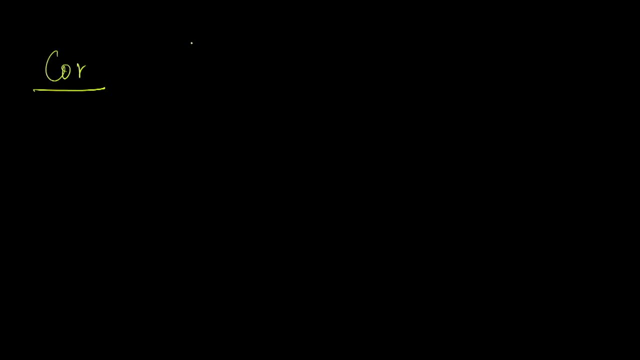 equinumerous with any smaller natural number. Therefore, as a corollary, we can argue that any set equinumerous with a proper subset of itself has to be infinite. In other words, it is not equinumerous with any natural number. 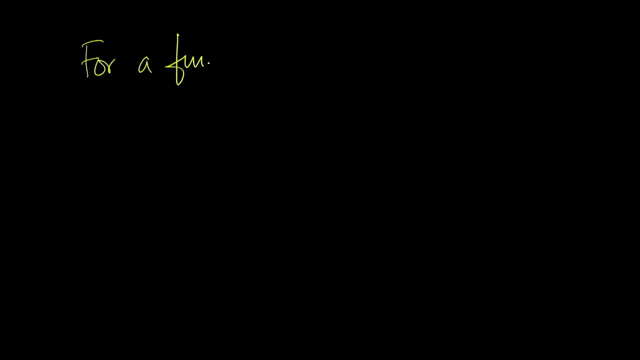 For a finite set, A. The natural number that is equinumerous with a is called the cardinal number of A. This is denoted as card A. For example, consider this set: This is equinumerous with 4. There. 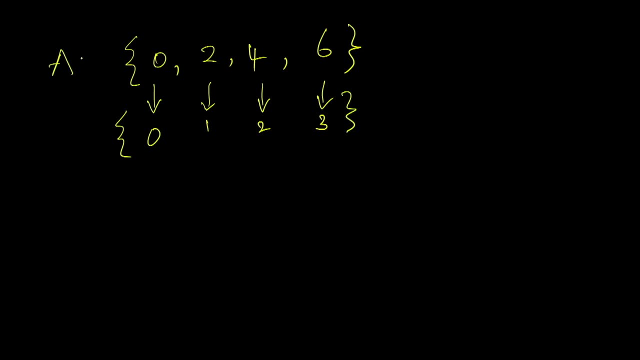 is a one-to-one mapping from the given set A onto the natural number 4.. Therefore A is equinumerous with 4.. In other words, the cardinal number of A is 4, or we say the cardinality of A is 4.. So for every finite set there is a natural number that forms its cardinality. 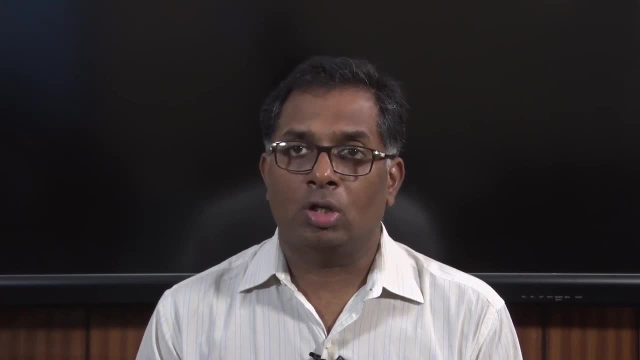 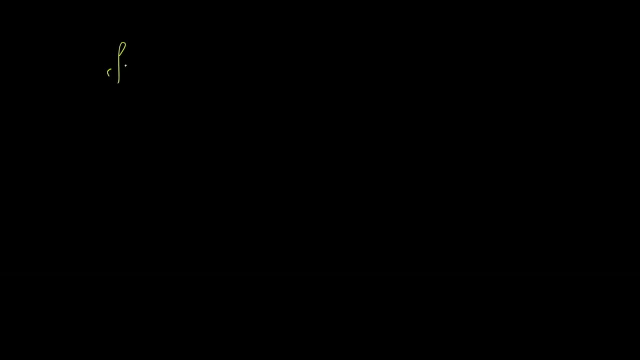 Two finite sets are equinumerous means they have exactly the same cardinal numbers. Or, in general, for any two sets, A and B, finite or infinite, we say that the cardinality of A is equal to cardinality of B. By the definition of cardinality, this is if, and only if, A is. 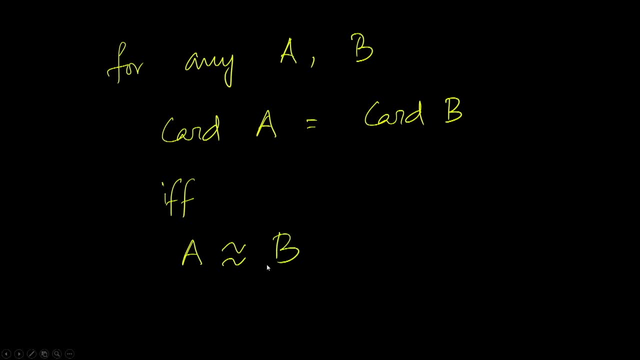 equinumerous with B, So there is a one-to-one onto mapping from A to B. that is precisely when the cardinality of A and B are identical. The cardinality of the set of natural numbers is denoted as Aleph nuot, Using the Hebrew. 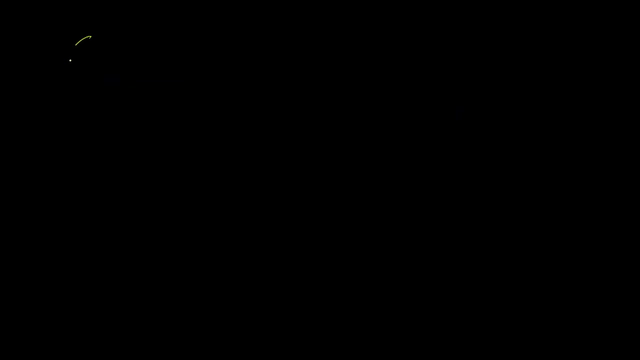 letter Aleph. Using cardinal numbers, we can form what is called cardinal arithmetic. Cardinal arithmetic has several interesting properties If kappa and lambda are cardinal numbers, which means there is a set A with cardinality kappa and there is a set B with cardinality lambda, or 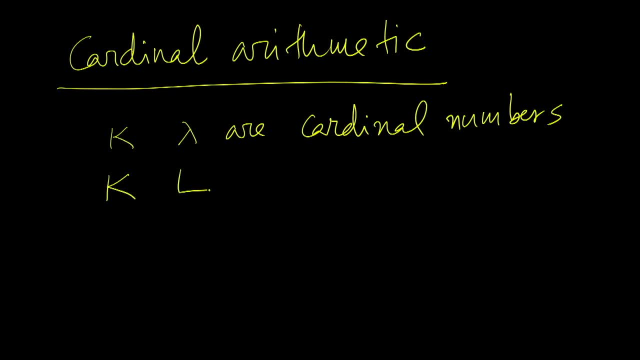 let us say, using matching letters k and l, with cardinalities kappa and lambda respectively. Then kappa plus lambda is the cardinal number of k- k union. l Kappa into lambda is the cardinal number of k cross. l Kappa power lambda is. 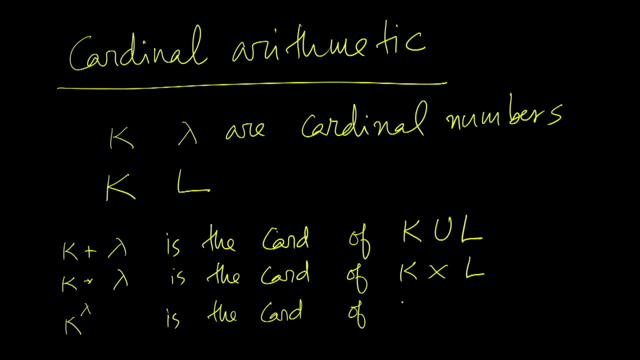 the cardinal number of k plus, So set of all functions from l to k. When k and lambda are finite, these of course function the way we expect. For example, if k and l are finite, sets k union. l has k plus lambda elements at the most. if k and l are disjoint, sets k into lambda is the. 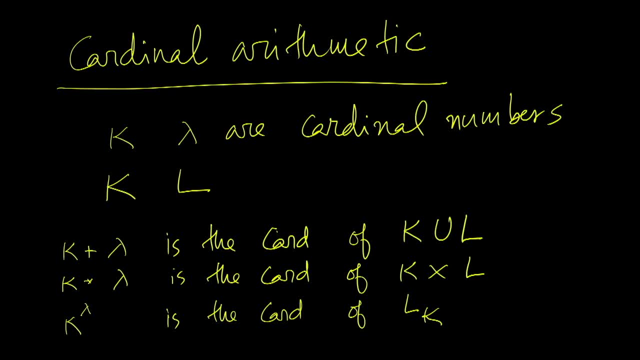 cardinality of k cross l, which is indeed the case. K has kappa elements and lambda log qua kalpa plus k. Didn't I say 1 minus k plus lambda is a nice part of this, but in, oh sorry, make some some exceptions. coming The right carries into k cross l plus k plus. 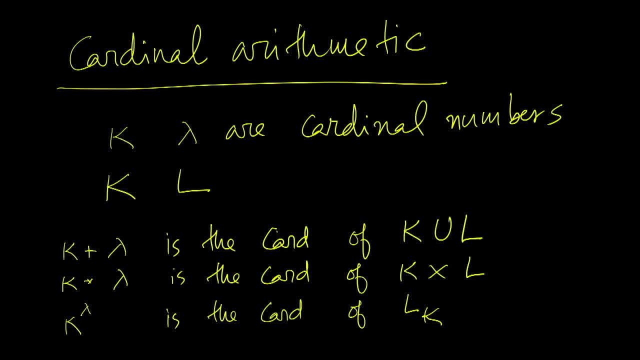 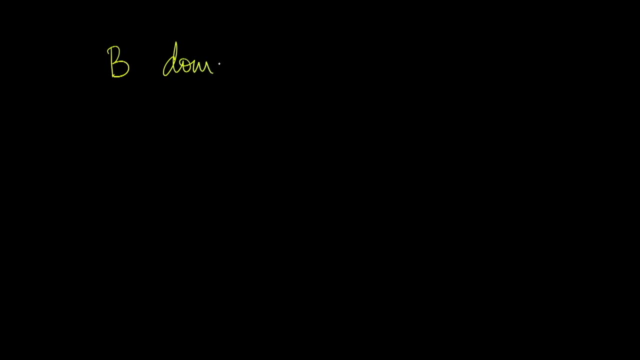 L has lambda elements. So kappa into lambda is the cardinality of k, cross L, kappa power. lambda is the cardinality of L to k. that is the set of all functions from L to k. We say that set B dominates A, which was denoted as in this fashion for two sets, A and B. we 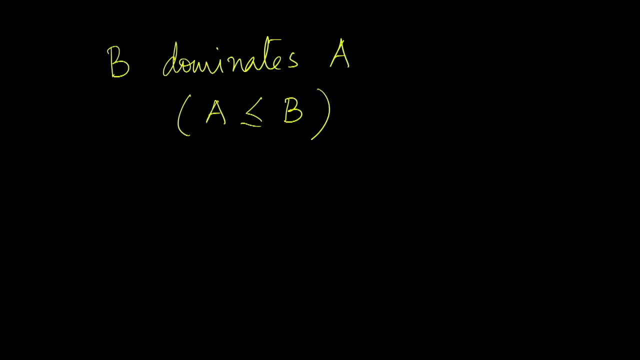 write A less than or equal to B to indicate that B dominates A. We say this precisely when there is a one to one mapping from A into B. So, mind you, this is an into mapping, Which means the cardinality of A is less than or equal to the cardinality of B. So, using 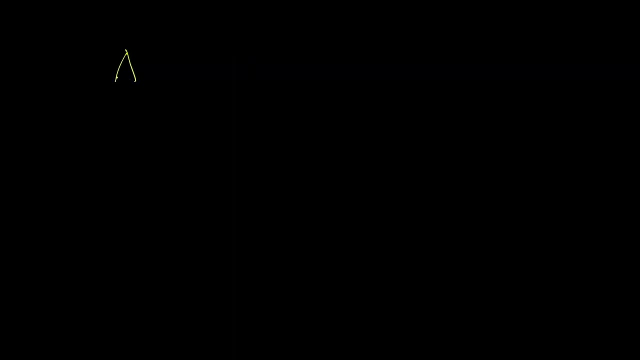 this definition, we can say that A is countable if, and only if, A is dominated by the set of natural numbers. In other words, the cardinality of A is less than or equal to the set of natural numbers. So the cardinality of A is less than or equal to the cardinality of L f naught. 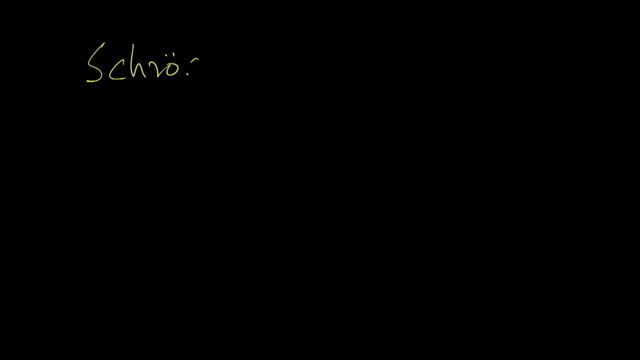 A famous theorem of set theory called Schroeder Bernstein theorem says that if B dominates A and A dominates B, then A and B are equinumerous. In other words, if the cardinality of A and B have this property that the cardinality of A is less than or equal to the cardinality, 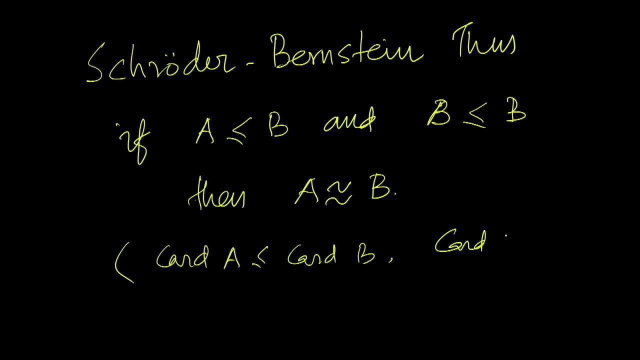 of B And the cardinality of B is less than or equal to the cardinality of B and A is equal to the cardinality of B, then B dominates A. So these 2 terms are very important. the 2 compartions are remains under. 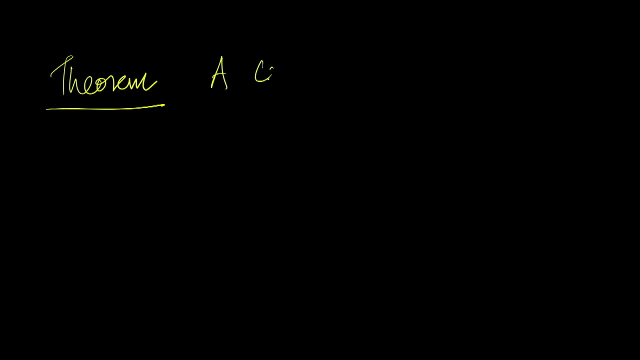 At a program what you do on a set of set of A and B. Yeah, Perieni, interval in between A and B. Yeah, So for a function a set of set of A is less than or equal to the cardinality of A, then the two have identical cardinality. 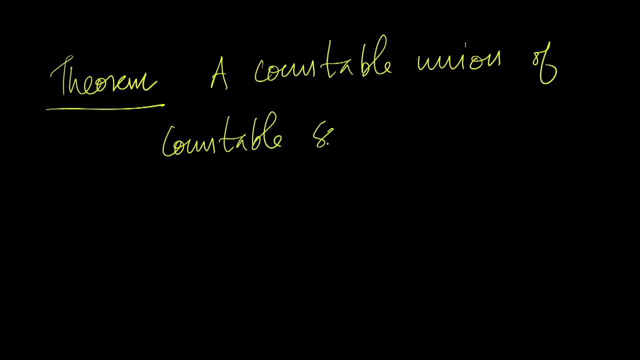 Related theorem is that a countable union of countable sets, solche set of A hyperspecificятive. Another theorem asserts that for a cardinal number, kappa, kappa is less than Lf naught if, and only if, kappa is finite. In other words, in a sense, the set of natural. 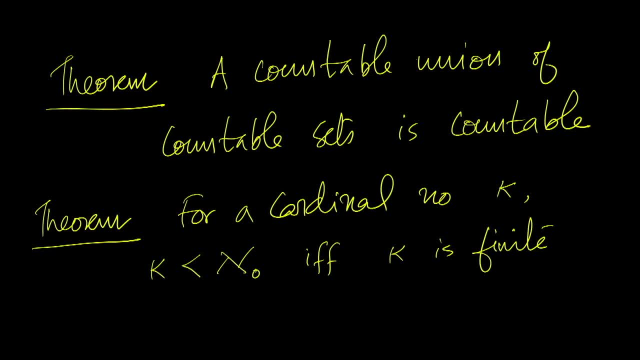 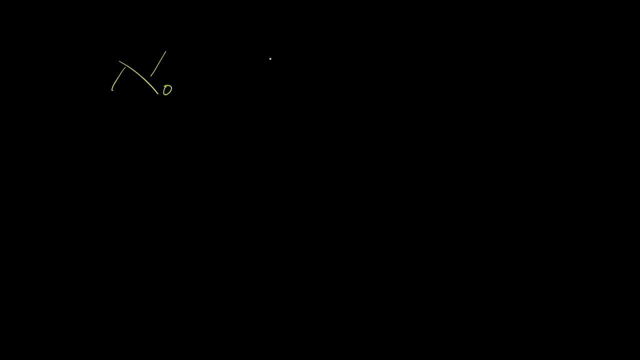 numbers is the smallest infinite set. So we know that Lf naught and 2 power Lf naught are not identical. Lf naught is the cardinality of the set of natural numbers and 2 power Lf naught is the cardinality of the set of all real numbers. We know that this is a countable 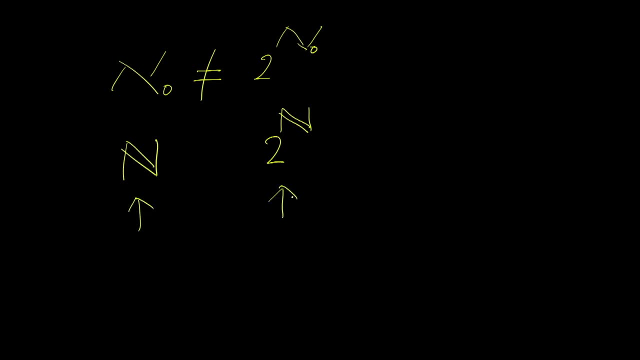 set and this is not a countable set. So the two have different cardinalities. but can there be a cardinality between them In these two? Cantor conjectured that there is no set of cardinality between Lf naught and 2 power Lf naught. This conjecture was called the continuum hypothesis In 1939,. 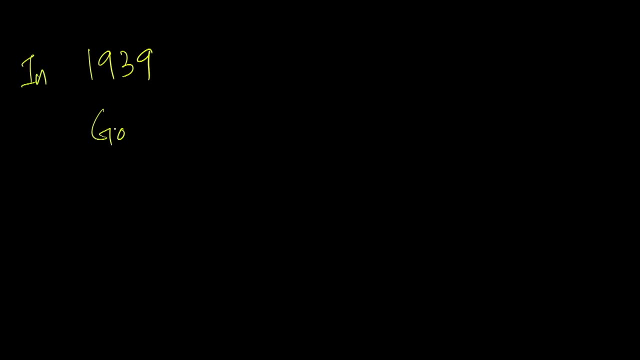 in 19 eleventh century, Gyódale showed that the continuum hypothesis cannot be disproved from the semilouf wrangle axioms of set theorem. Ok Ok, Ok Ok. 1939, Gödel showed that continuum hypothesis cannot be disproved from the axiom subset.